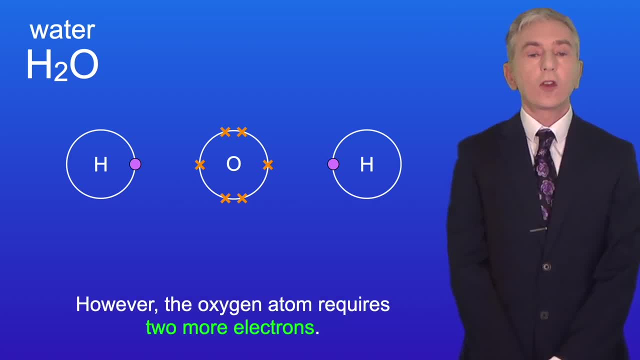 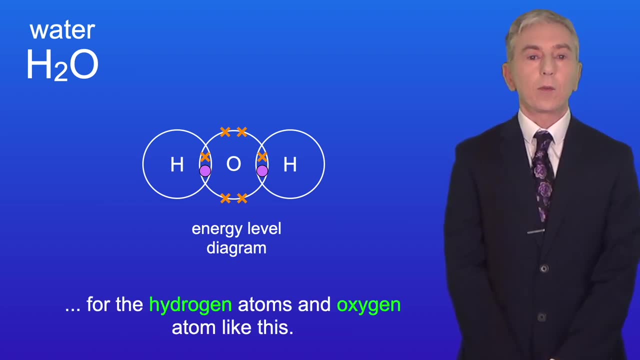 achieve a full outer energy level. However, the oxygen atom requires two more electrons. We can use this formula for the hydrogen atoms. an oxygen atom like this, By sharing electrons. both the hydrogen atoms and the oxygen atom have a full outer energy level. Remember that a shared pair of 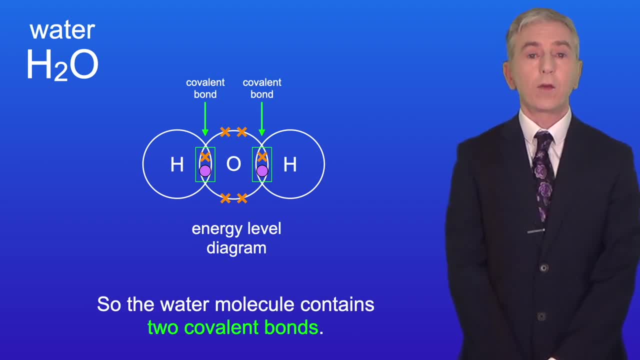 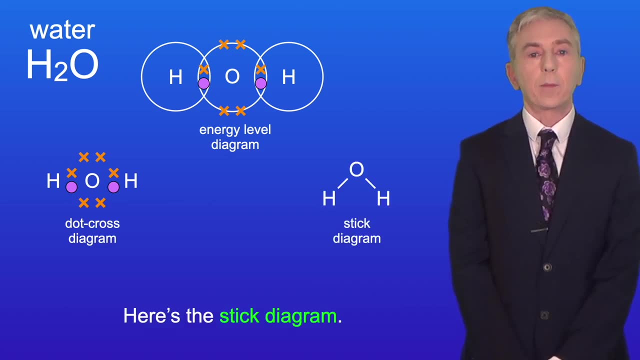 electrons is a covalent bond, So the water molecule contains two covalent bonds. Here's the dot and cross diagram for the water molecule and here's the stick diagram. And remember that in a stick diagram a single line represents a single covalent bond. 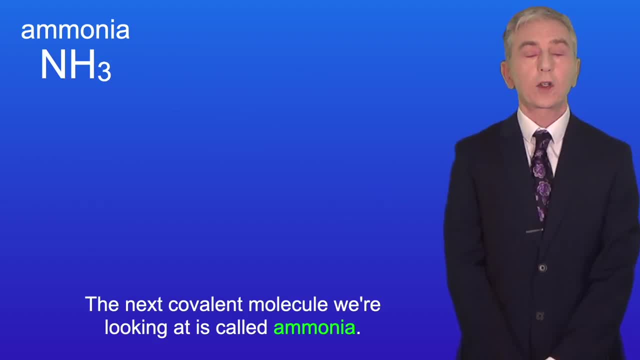 OK, the next covalent molecule we're looking at is called ammonia. Ammonia has a formula NH3. This tells us that an ammonia molecule contains one atom of nitrogen and three atoms of hydrogen. I'm showing you an atom of nitrogen here. Nitrogen has five electrons in its outer energy level. Hydrogen atoms only have one. 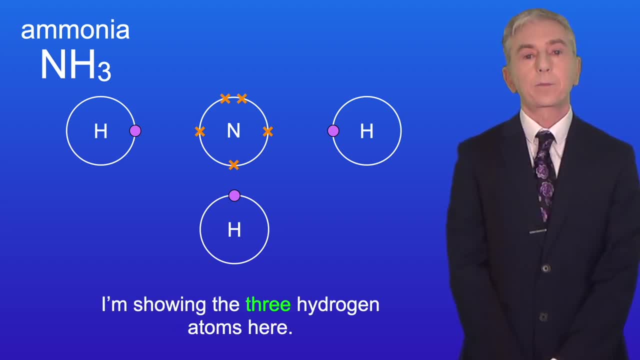 electron, and I'm showing the three hydrogen atoms here. I'd like you to draw the covalent bonding in the ammonia molecule. That includes the energy level diagram, the dot and cross diagram and the stick diagram. So pause the video now and try this yourself. OK, here's the energy level diagram for ammonia. We can. 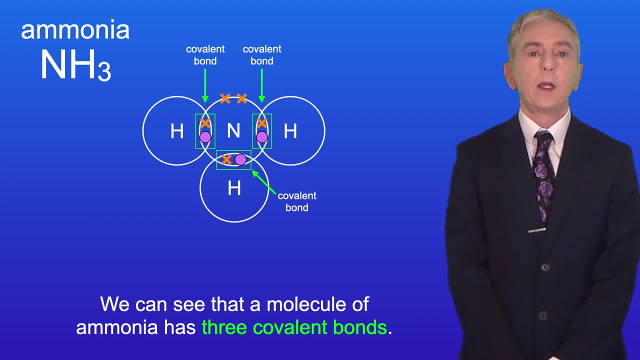 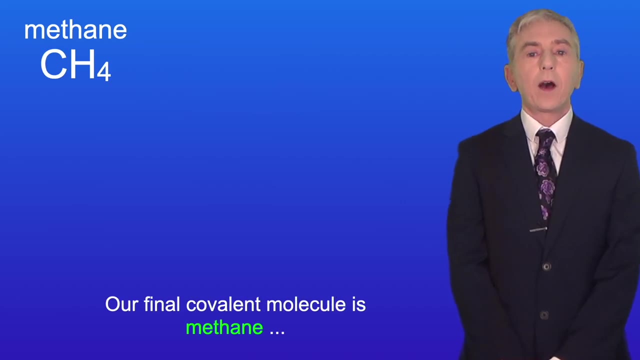 see that a molecule of ammonia has three covalent bonds. By sharing electrons, the nitrogen atom and the hydrogen atoms have each achieved a full outer energy level. Here are the dot and cross diagram. OK, our final covalent molecule is methane, which has the formula CH4. This tells us that a 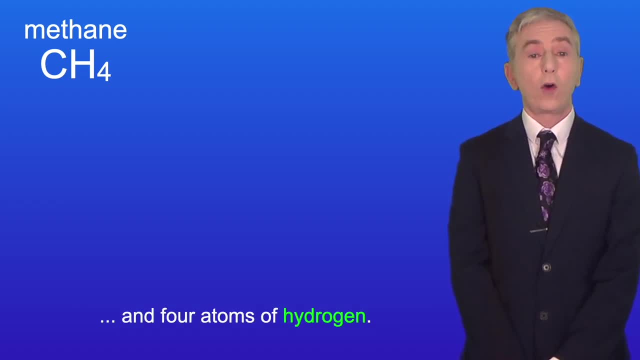 methane molecule contains one atom of carbon and four atoms of hydrogen. I'm showing you an atom of carbon here. Carbon has four electrons in its outer energy level. Here are the four hydrogen atoms, and remember that hydrogen only has one electron. I'd let you to draw the covalent bonding in the. 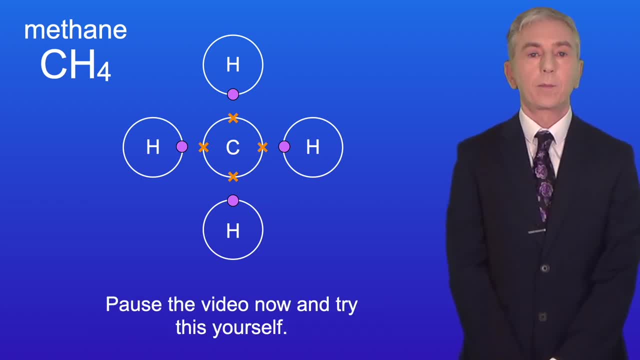 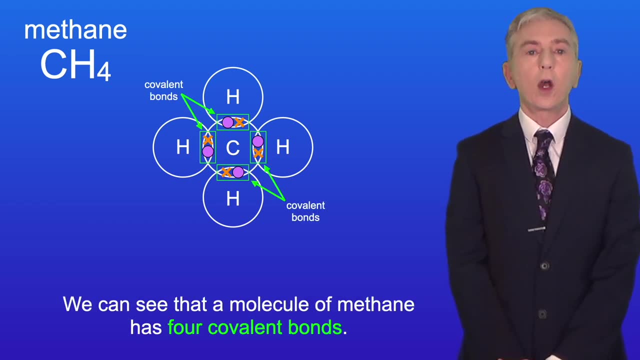 methane molecule. So pause the video now and try this yourself. OK, here's the energy level diagram for methane. We can see that a molecule of methane has four covalent bonds, And now the carbon atom and the hydrogen atoms all have full outer energy levels.